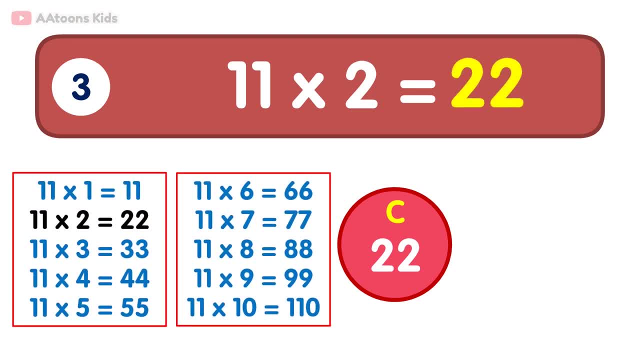 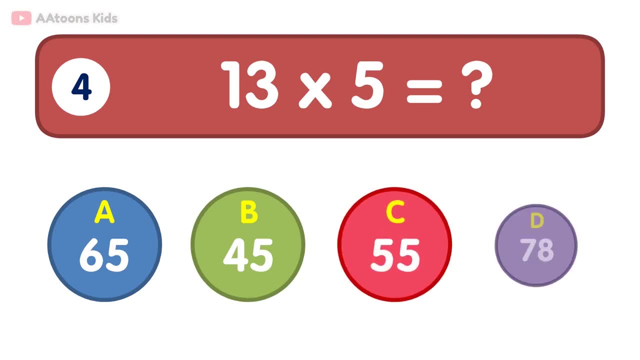 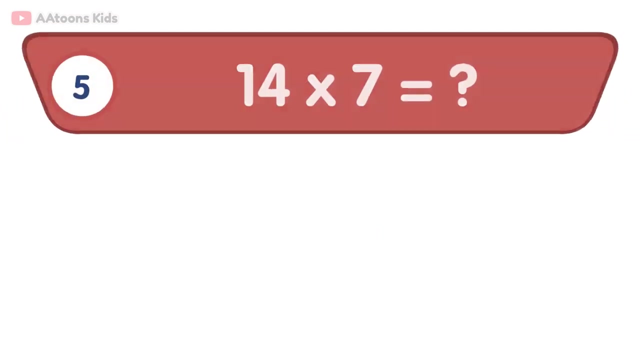 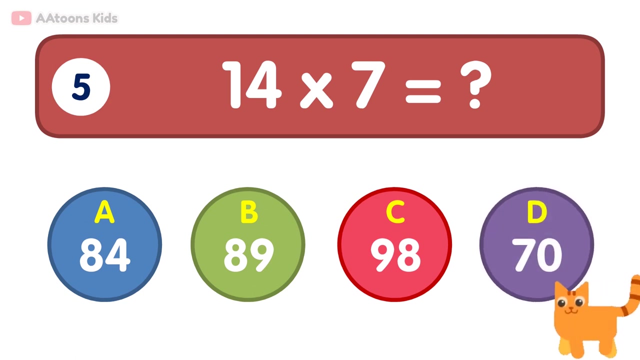 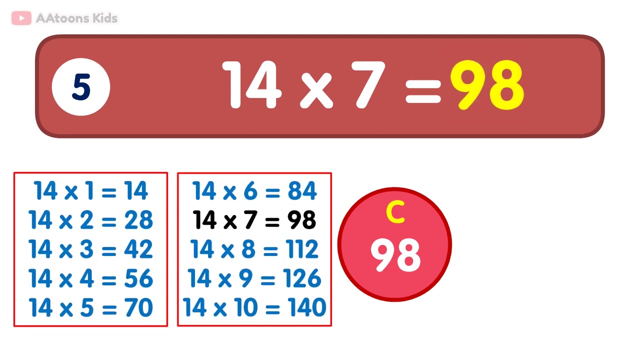 22.. 11 times 2 is 22.. 13 times 5 is equal to 65.. 13 times 5 is 65.. 14 times 7 is equal to 98.. 14 times 7 is 98.. 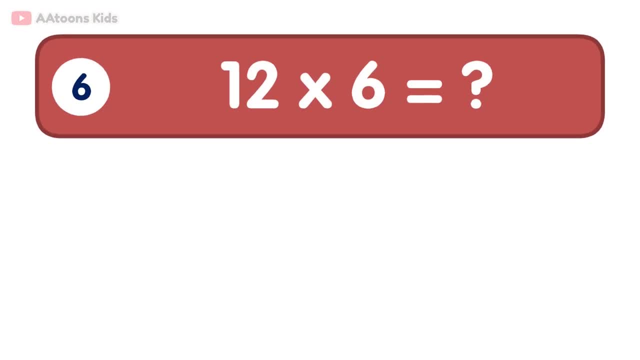 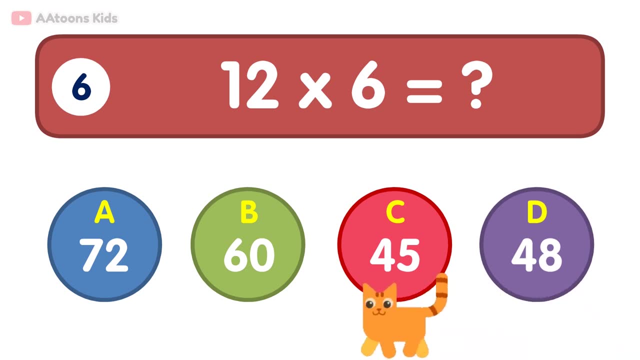 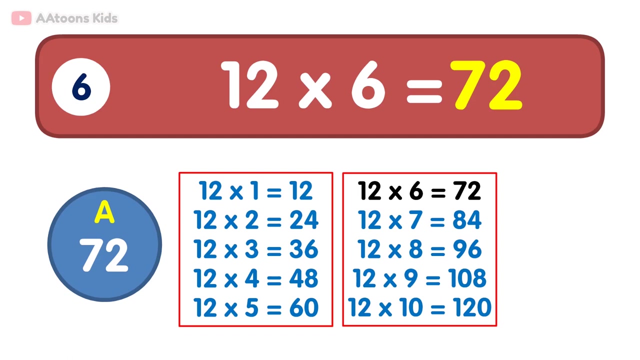 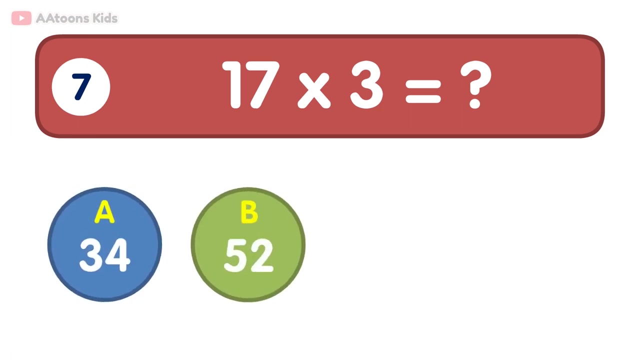 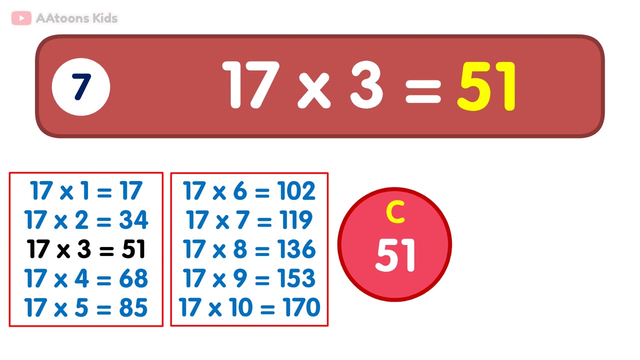 12 times 6 is equal to 12 times 6 is equal to 14 times 7 is equal to 12 x 6 is 72. 17 x 3 is equal to 51. 17 x 3 is 51. 15 x 8 is equal to. 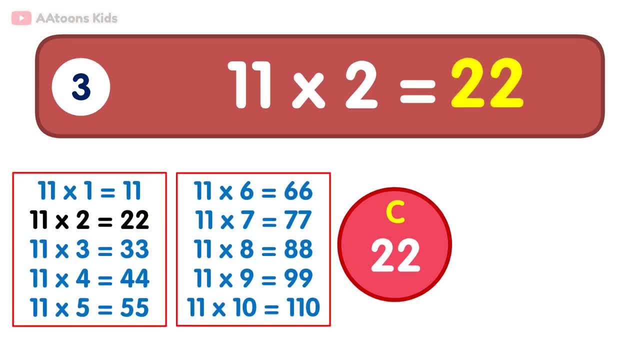 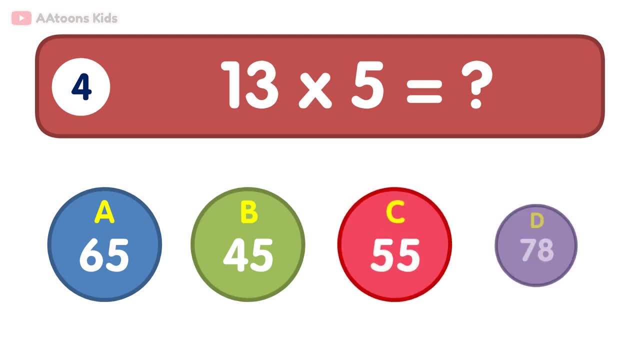 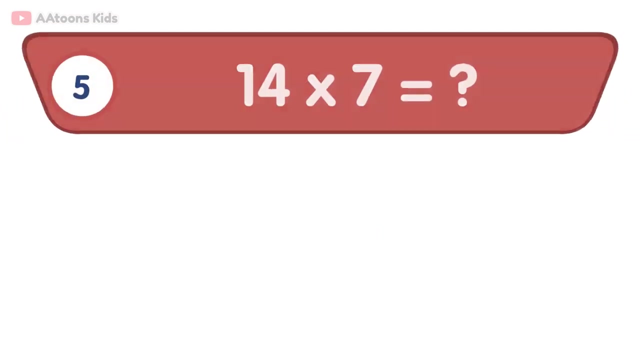 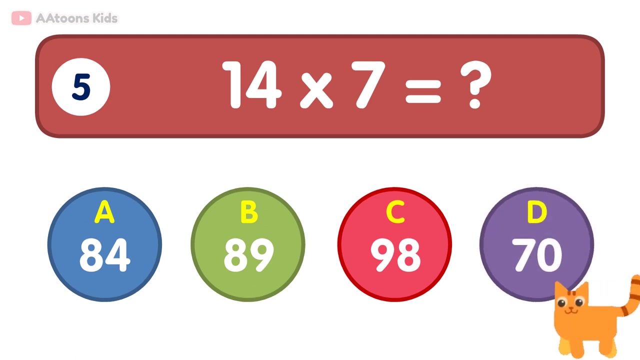 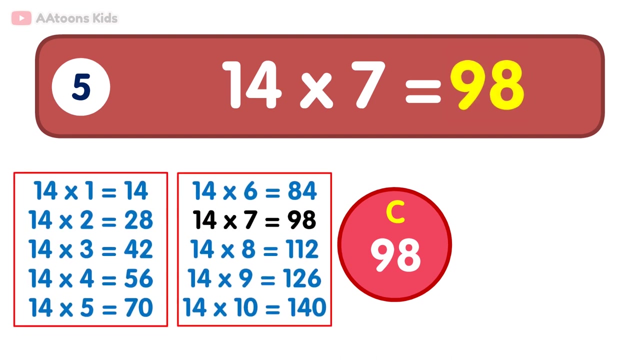 22.. 11 times 2 is 22.. 13 times 5 is equal to 65.. 13 times 5 is 65.. 14 times 7 is equal to 98.. 14 times 7 is 98.. 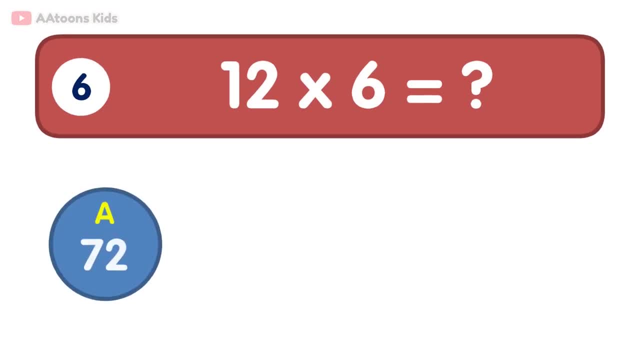 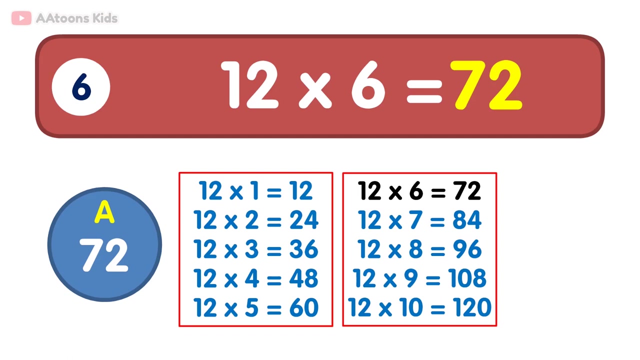 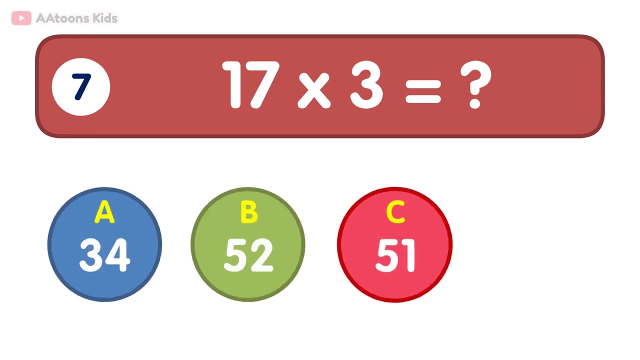 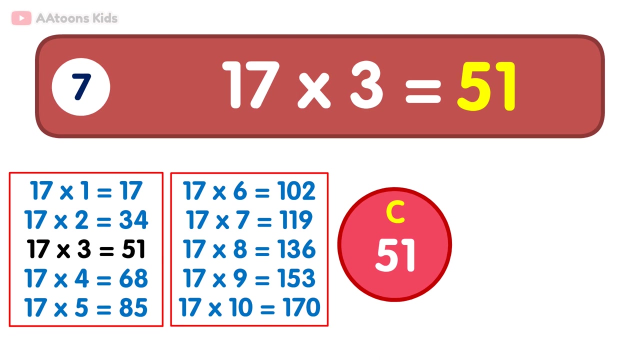 12 times 6 is equal to 16.. 14 times 7 is equal to 12 x 6 is 72. 17 x 3 is equal to 51.. 17 x 3 is 51. 15 x 8 is equal to. 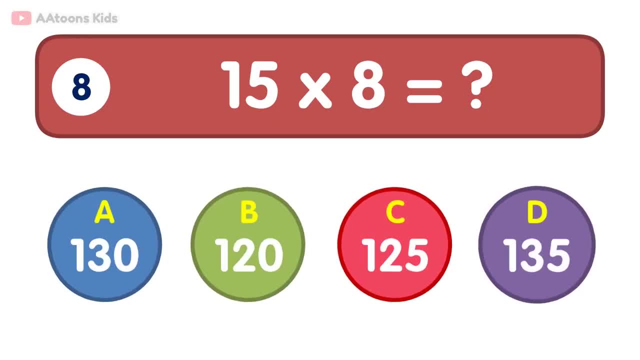 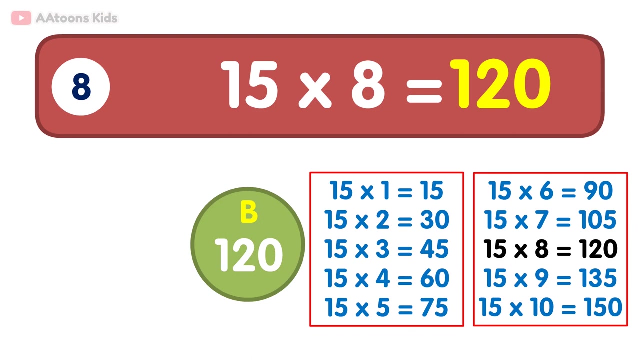 50.. 15 x 8 is equal to 50.. 15 x 8 is equal to 50.. 15 x 8 is equal to 120,. 15 times 8 is 120. 19 times 2 is equal to. 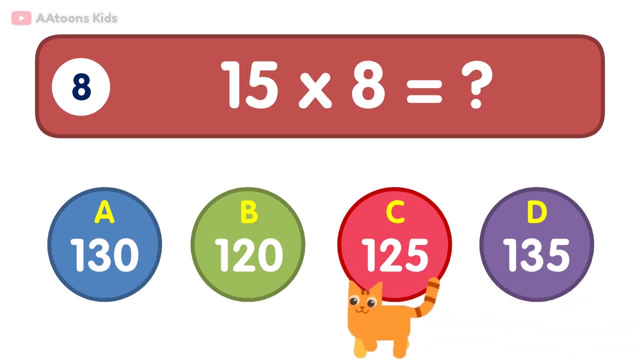 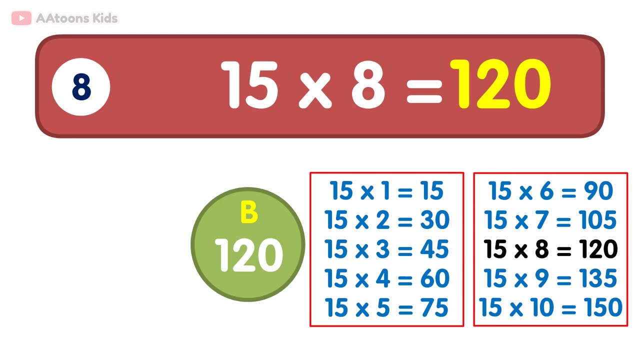 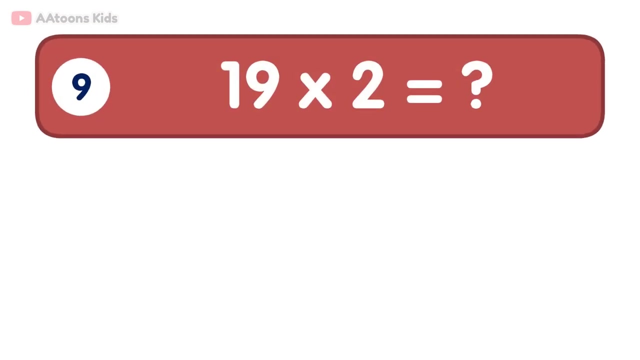 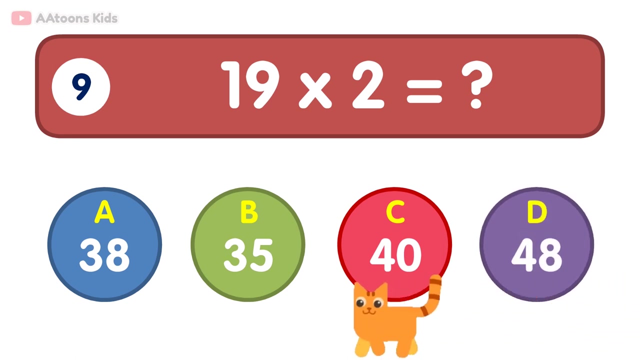 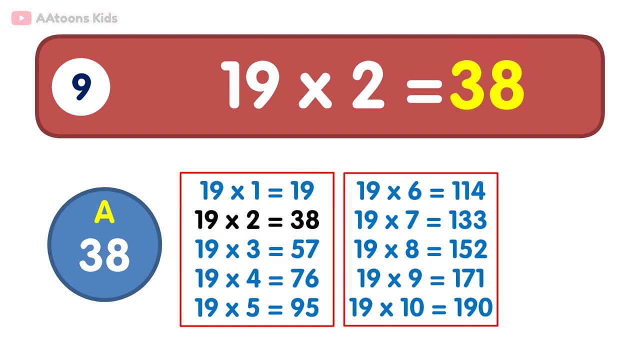 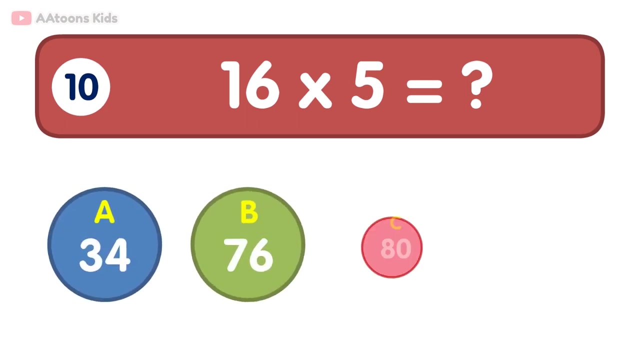 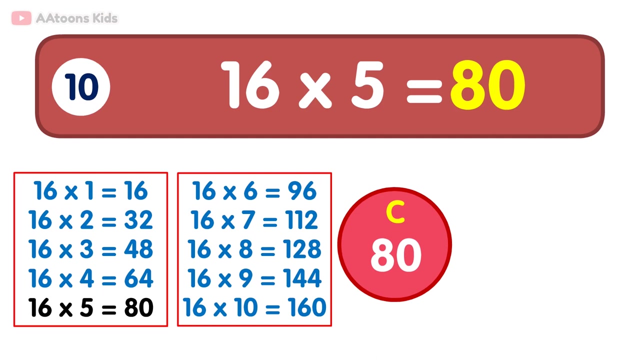 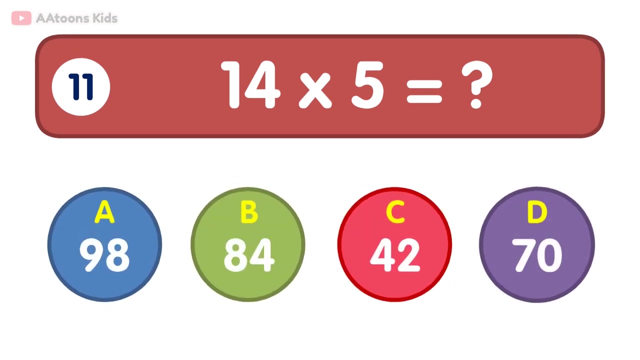 120. 15 x 8 is 120. 19 x 2 is equal to 30. 38. 19 x 2 is 38. 16 x 5 is equal to 30. 18, 16 x 5 is 18. 14 x 5 is equal to. 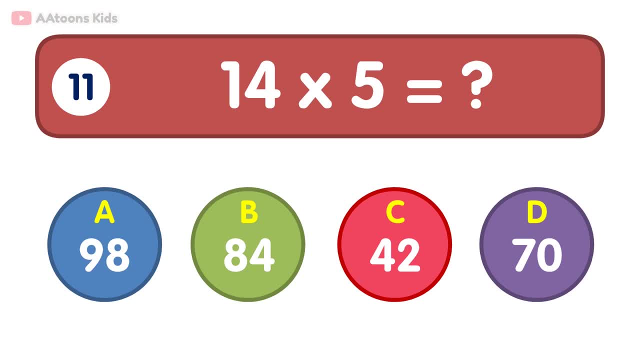 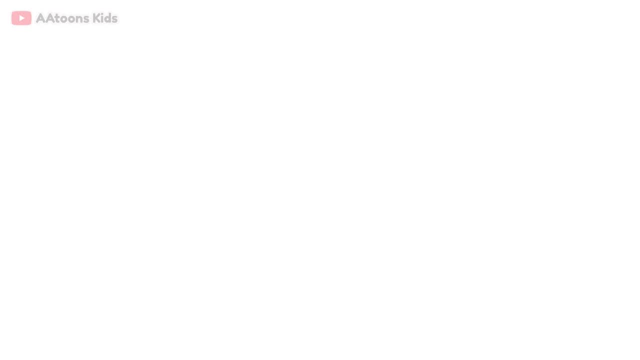 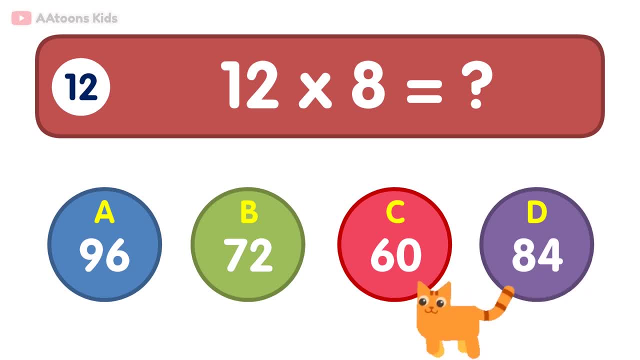 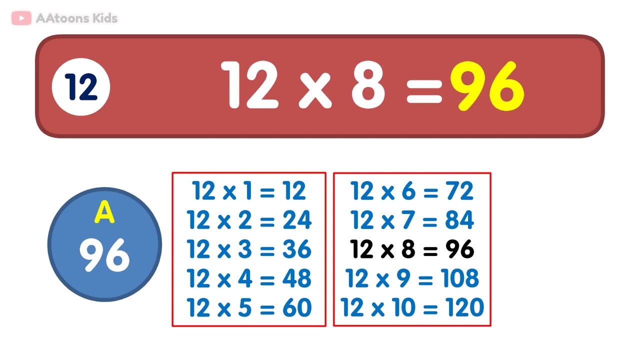 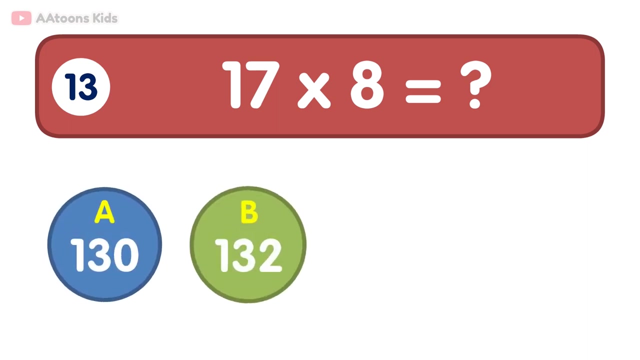 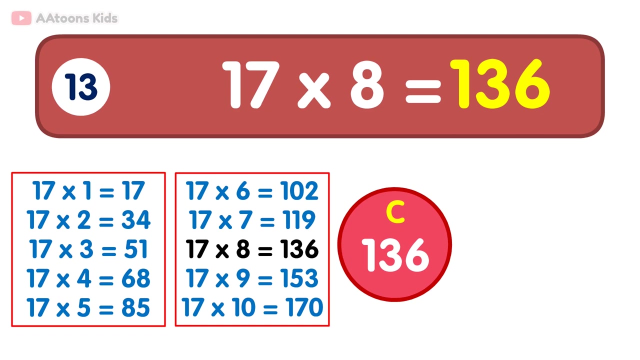 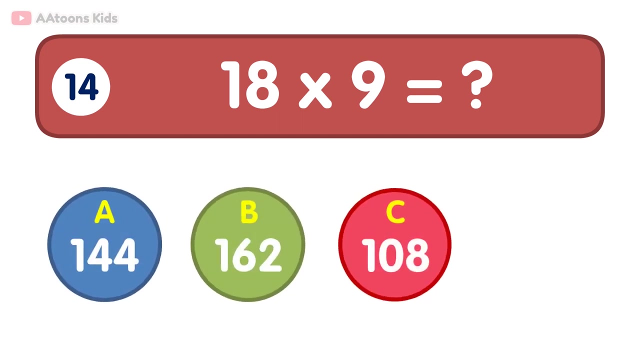 12 x 8 is equal to 11, 8, 9, 10, 10, 96.. 12 × 8 is 96.. 17 × 8 is equal to 136.. 17 × 8 is equal to 136.. 18 × 9 is equal to. 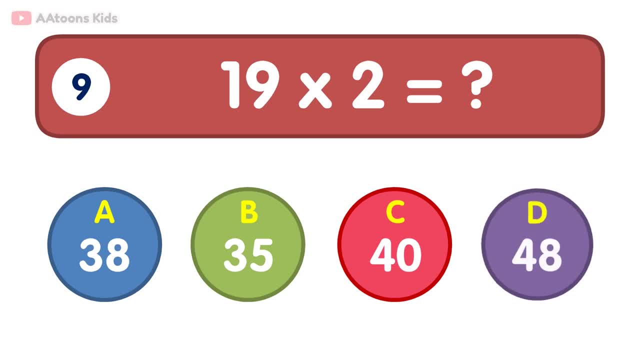 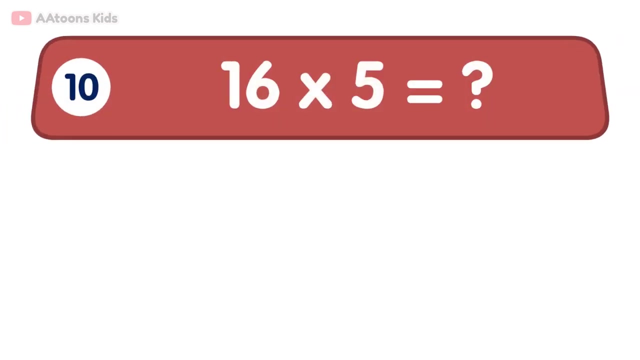 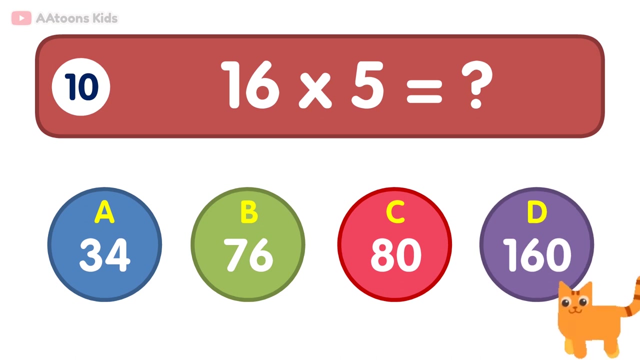 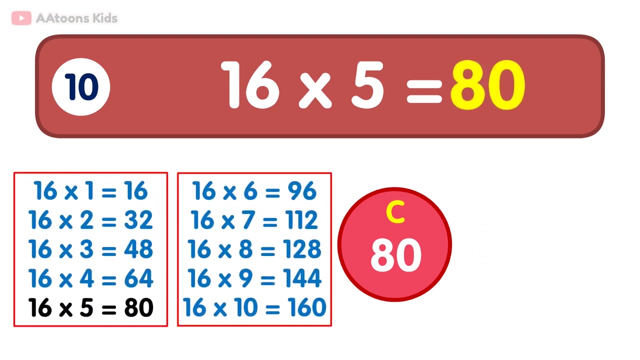 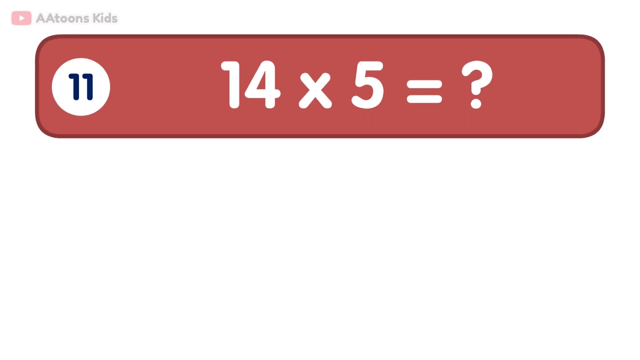 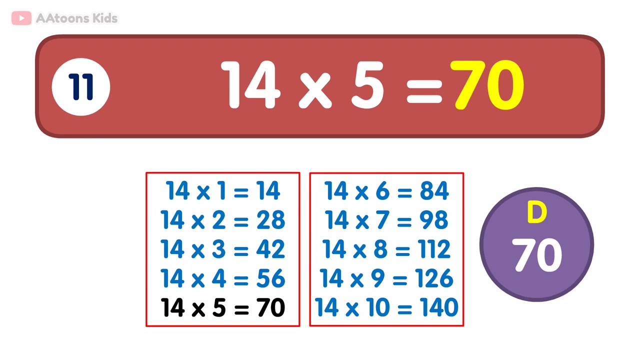 38, 19 times 2 is 38. 16 times 5 is equal to 57,, 58,, 59,, 60, 18.. 16 times 5 is 18.. 14 times 5 is equal to 17.. 14 times 5 is 70.. 12 times 8 is equal to. 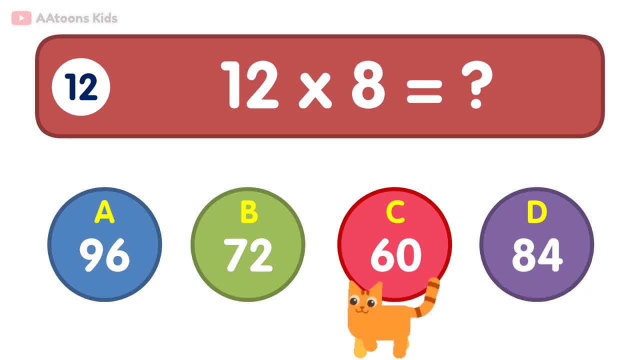 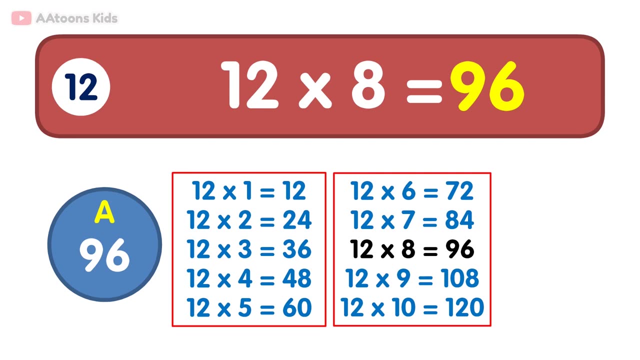 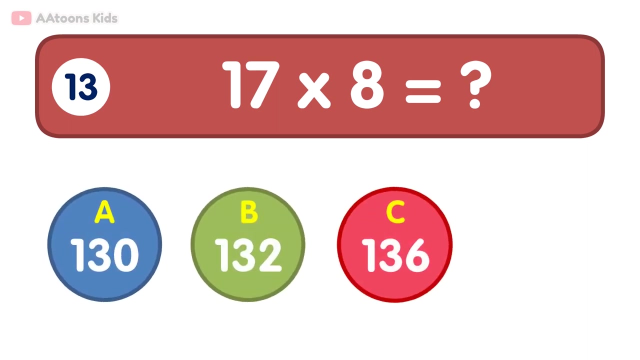 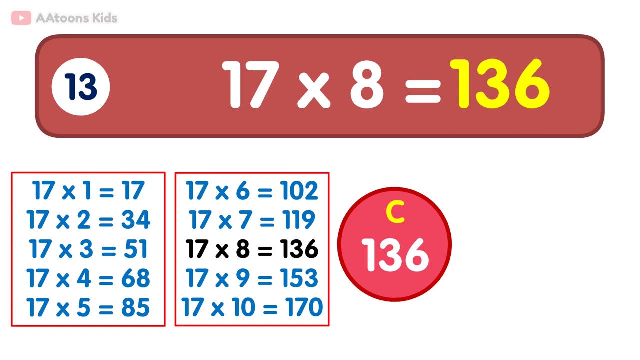 96.. 12 times 8 is 96.. 17 times 8 is equal to 99.. 12 times 8 is 96.. 17 times 8 is equal to 136.. 17 times 8 is 136.. 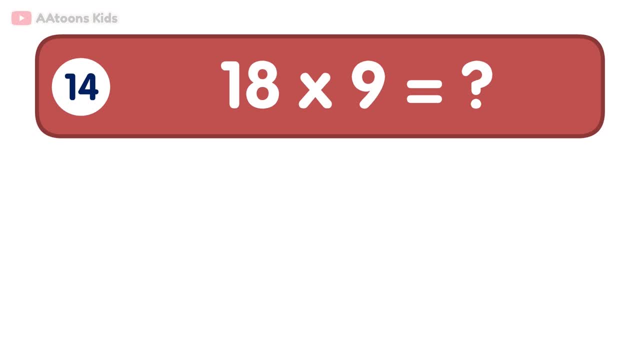 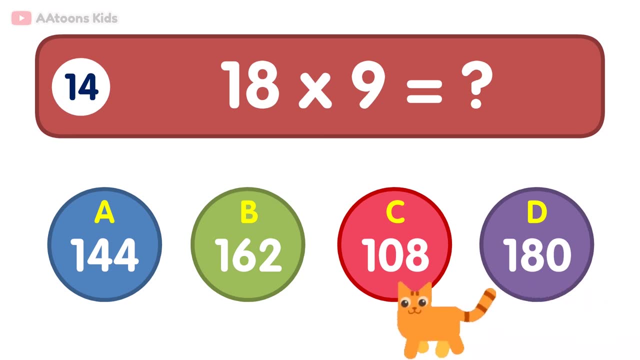 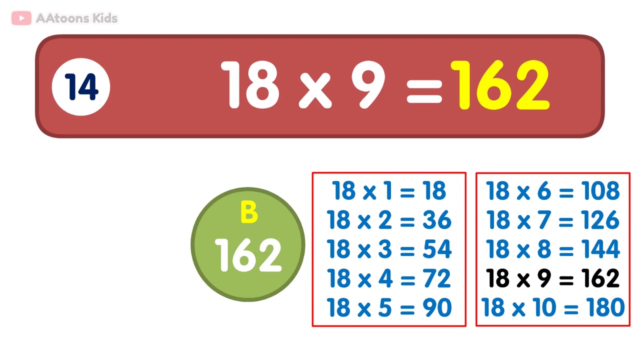 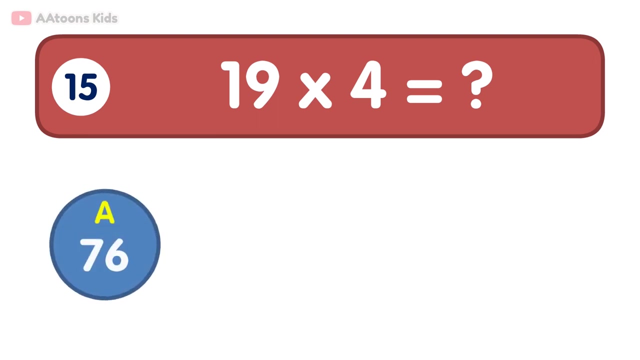 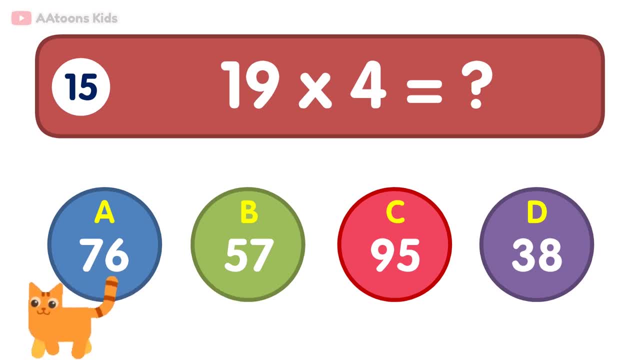 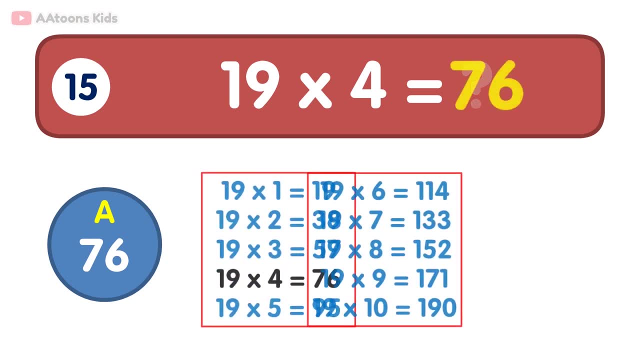 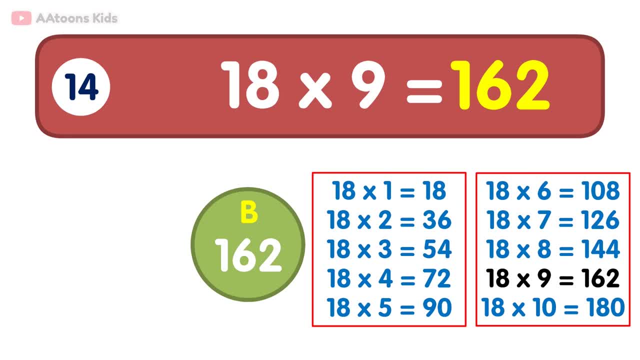 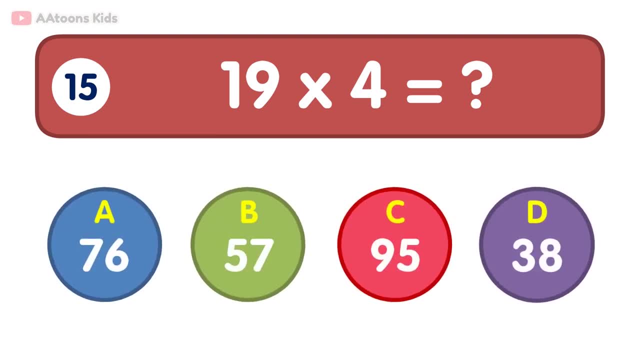 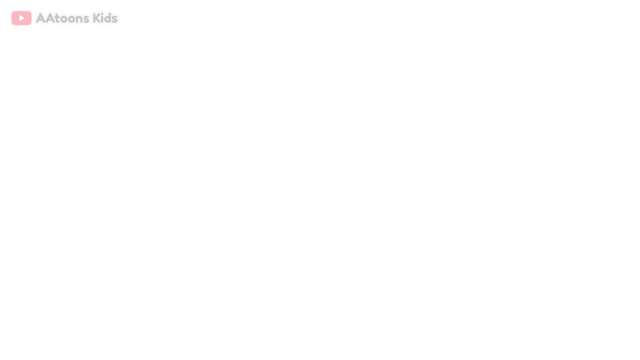 162.. 18 × 9 is equal to 162.. 19 × 4 is equal to 76.. 19 × 4 is equal to 76.. 20 × 3 is equal to 60.. 20 × 3 is equal to 64.. 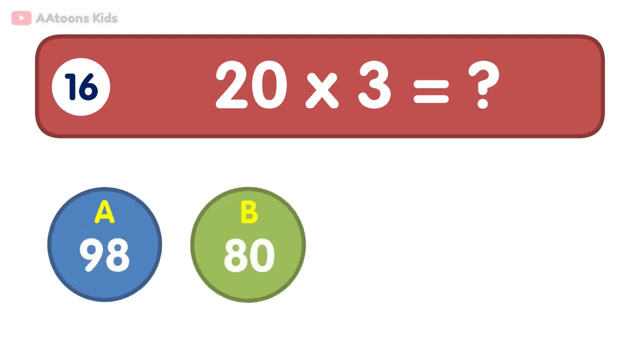 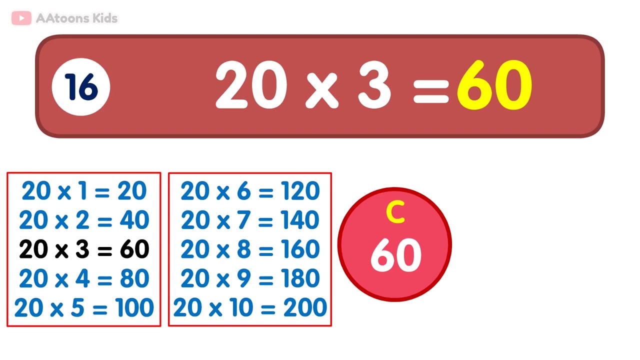 21 × 3 is equal to International�도. 20 × 3 is equal to 100.. 26 × 2 is equal to 40.. 24 × 3 is equal to unnecessary needed 1%, 27 × 4.. 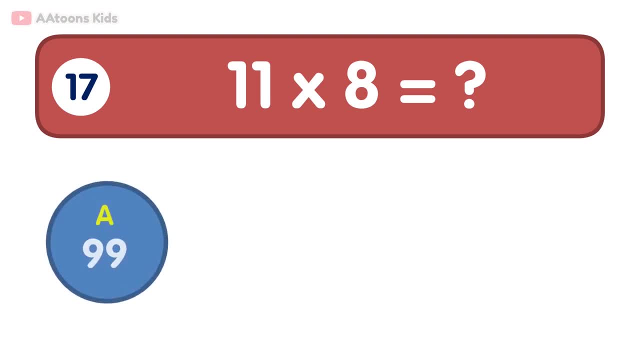 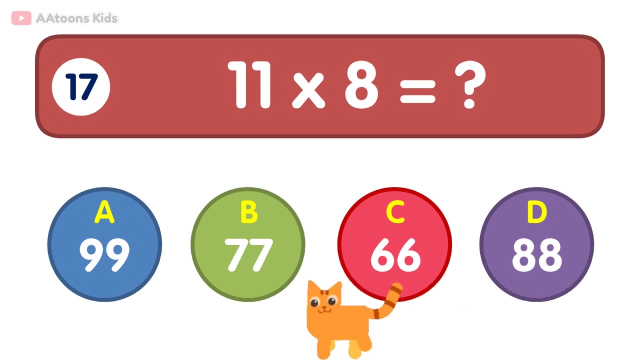 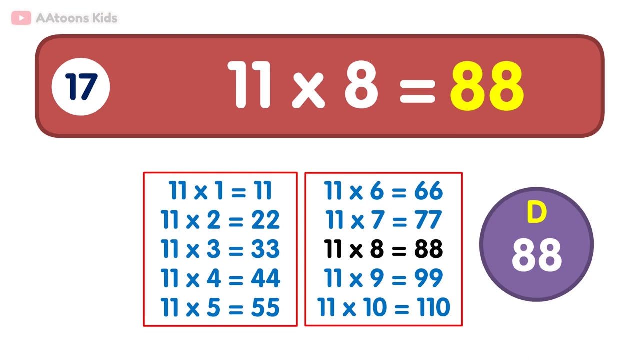 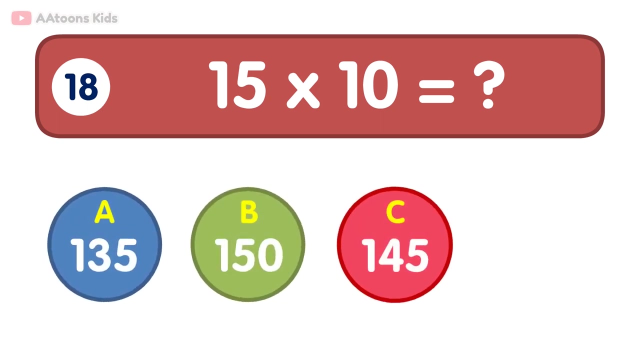 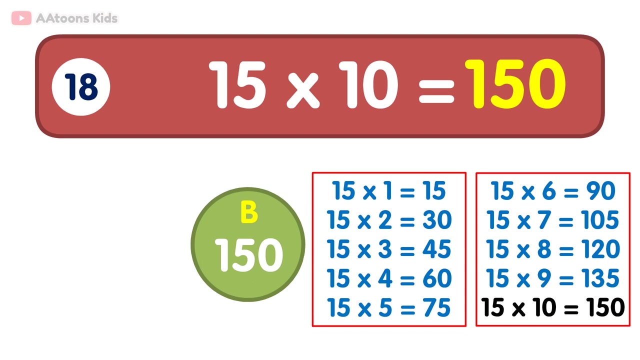 28 × 3 is equal to 40.. 88.. 11 times 8 is 88.. 15 times 10 is equal to 150.. 15 times 10 is 150.. 16 times 9 is equal to. 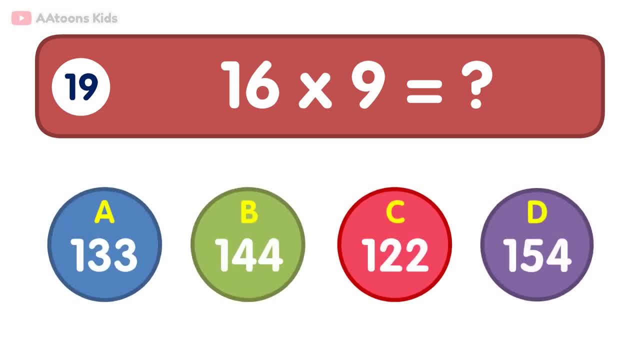 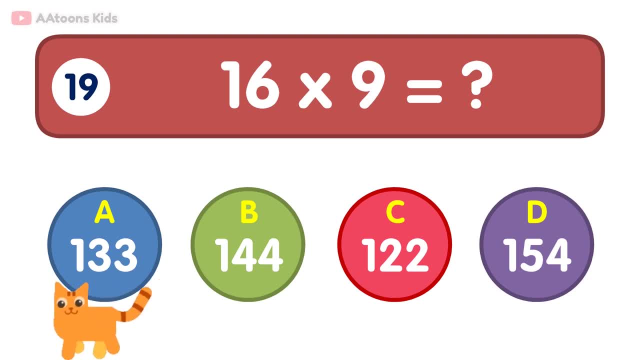 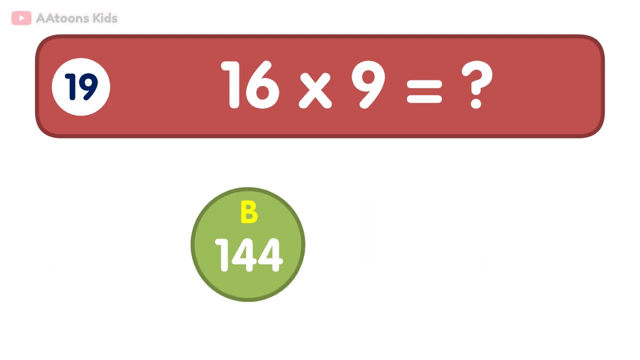 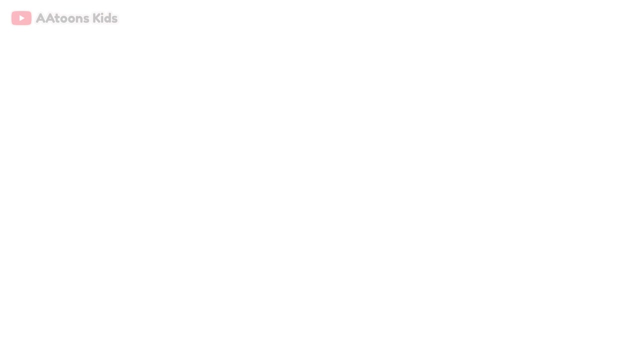 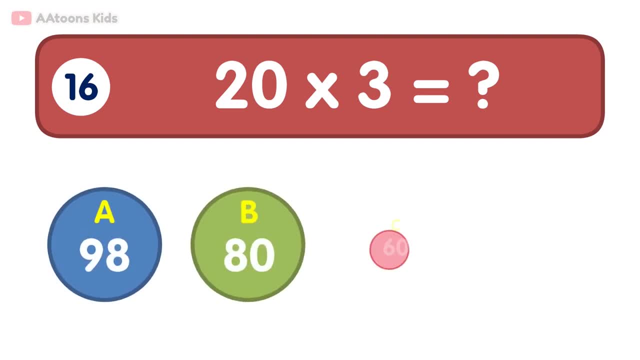 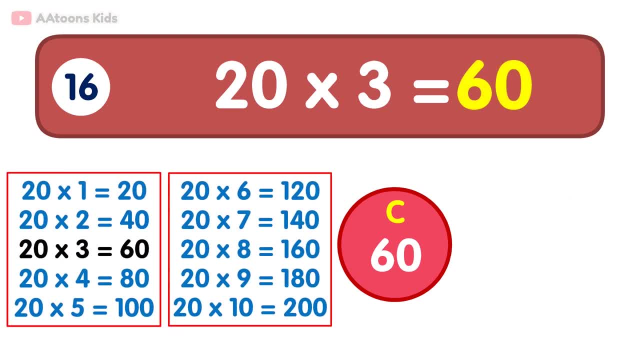 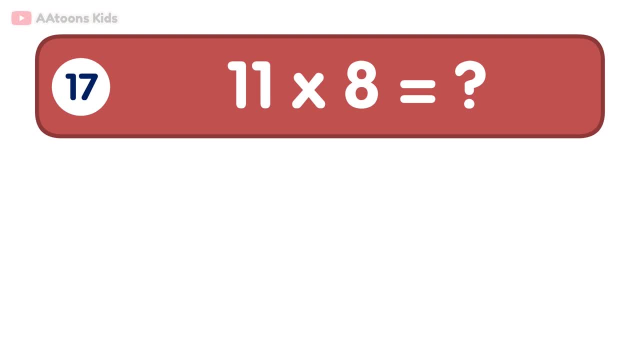 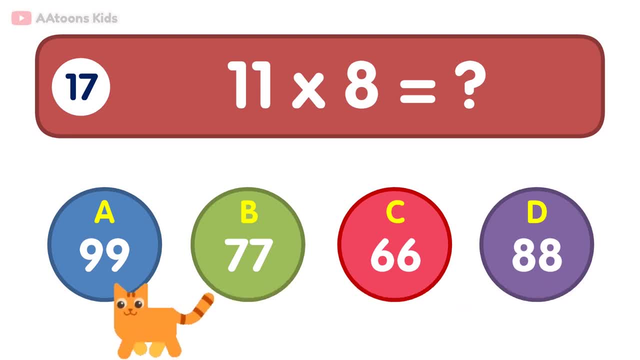 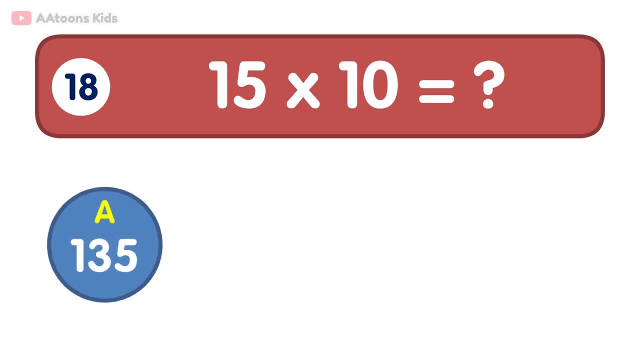 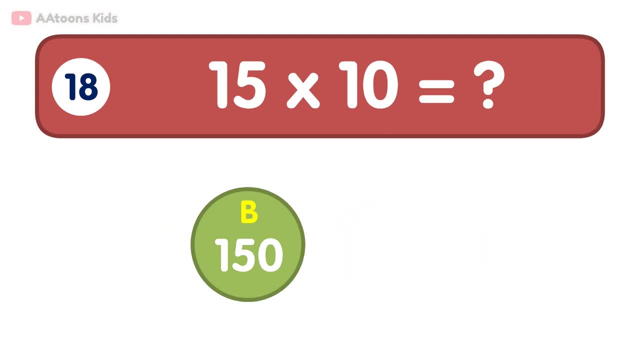 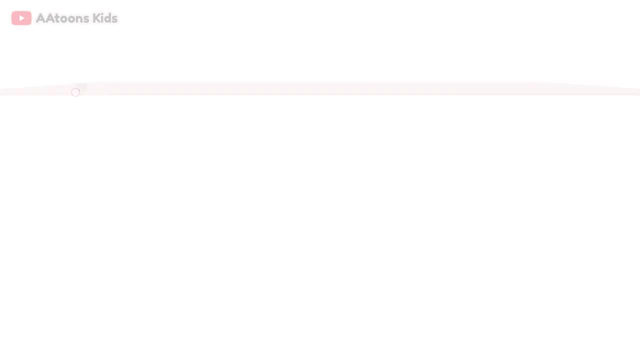 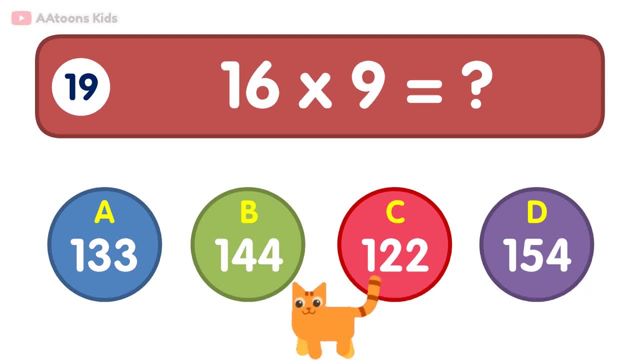 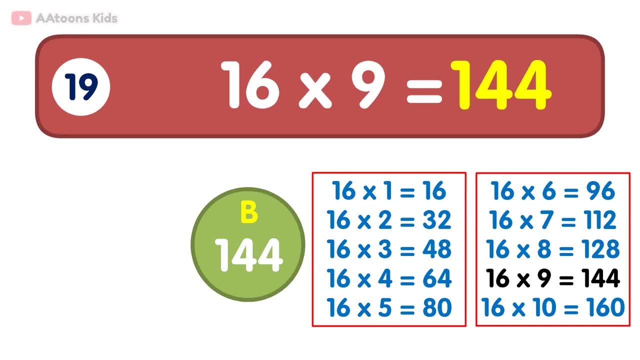 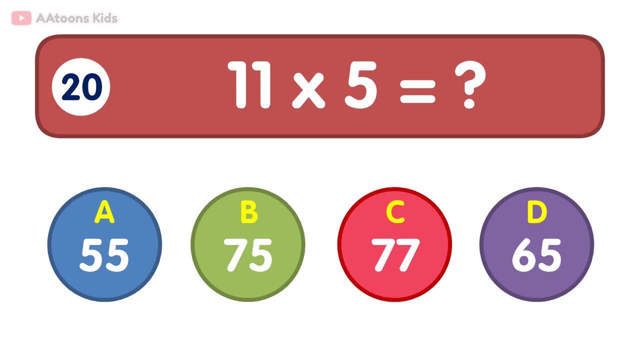 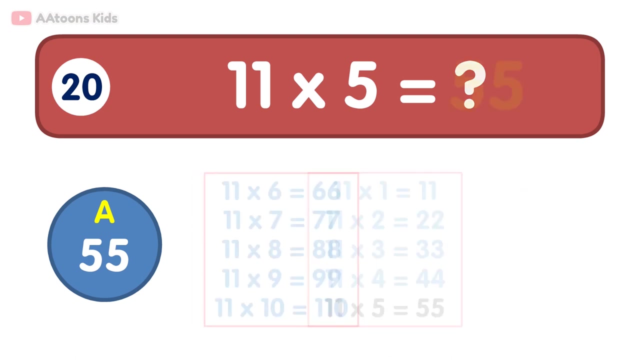 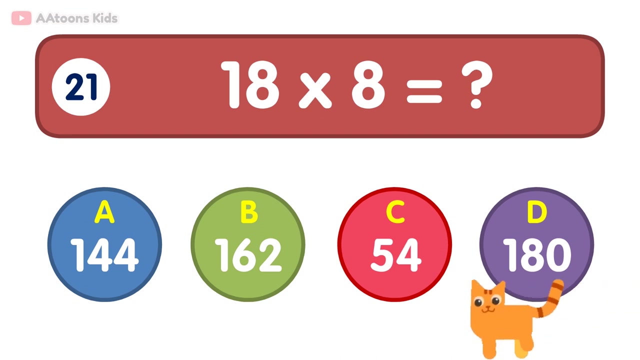 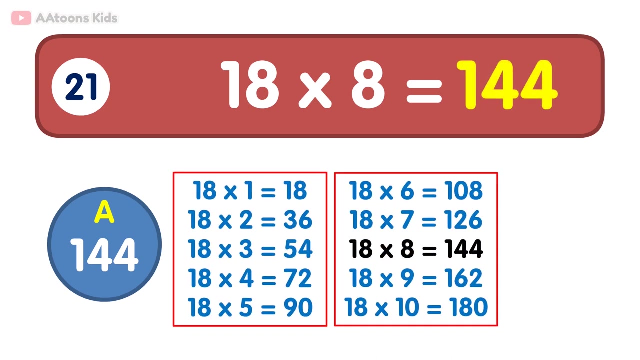 1. 1. 1. 1. 11 times 5 is equal to 55. 11 times 5 is 55. 18 times 8 is equal to 144. 18 times 8 is 144. 11 times 8 is equal to 15. 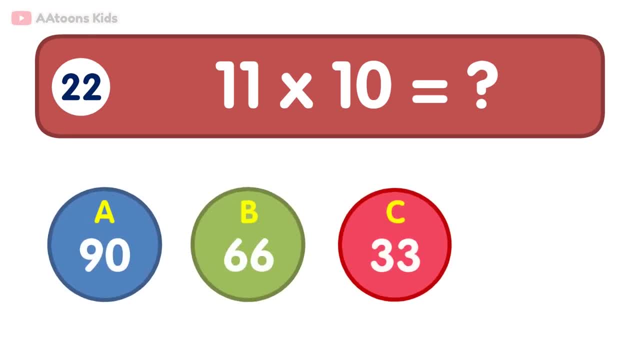 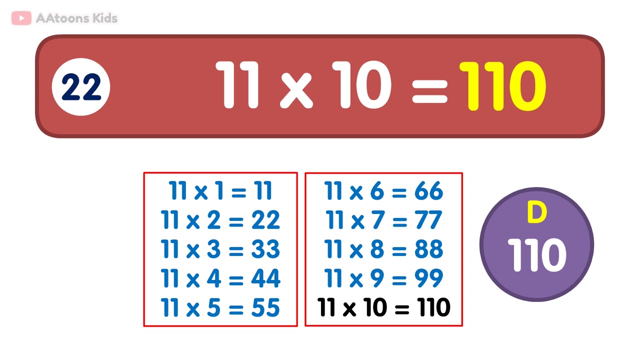 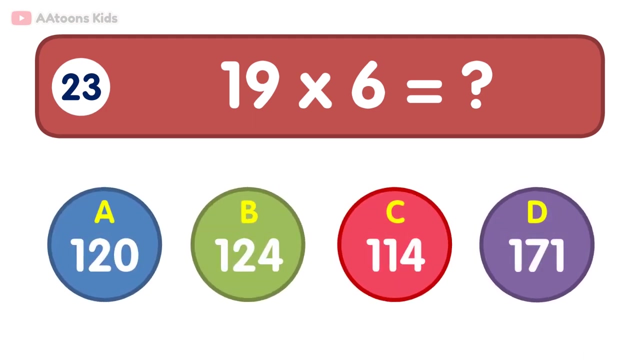 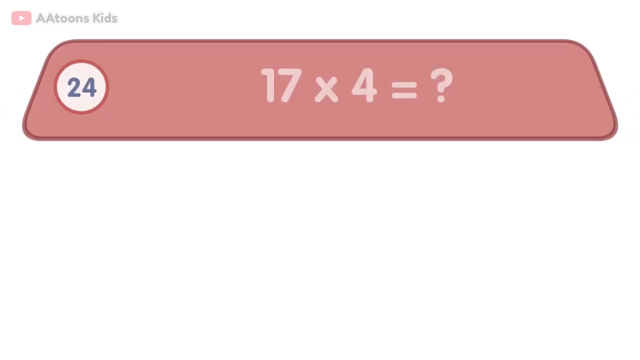 11 times 10 is equal to 10. 11 times 10 is 110. 19 times 6 is equal to 5. 15 times 6 is equal to 5. 19 times 6 is equal to 5: 114,. 19 times 6 is 114. 17 times 4 is equal to. 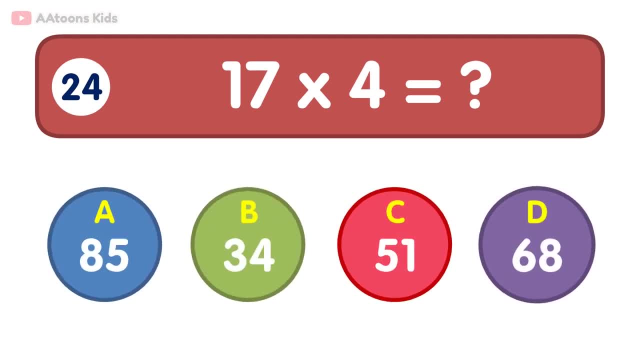 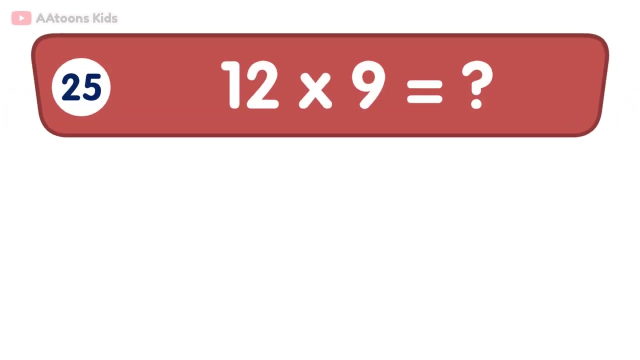 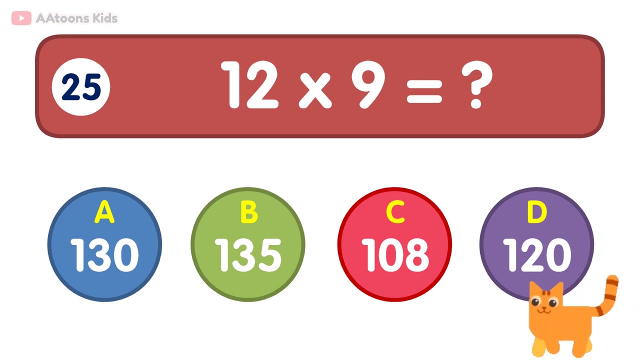 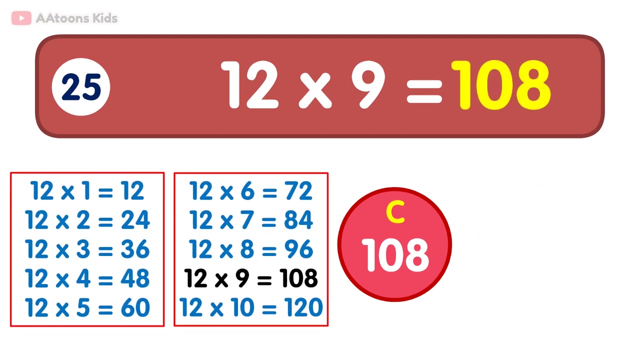 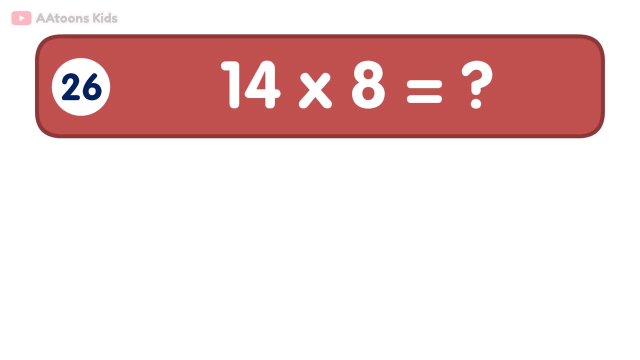 68.. 17 times 4 is 68.. 12 times 9 is equal to 12 times 9 is equal to 12 times 9 is equal to 108,. 12 times 9 is 108. 14 times 8 is equal to. 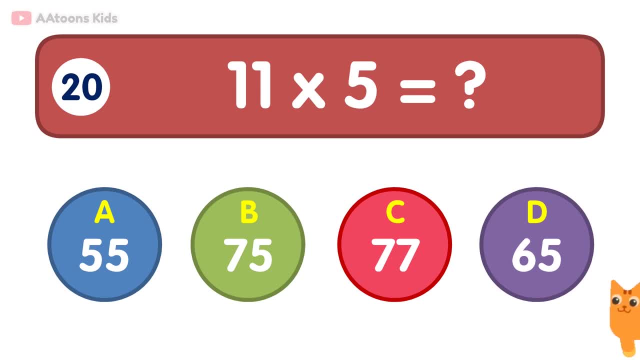 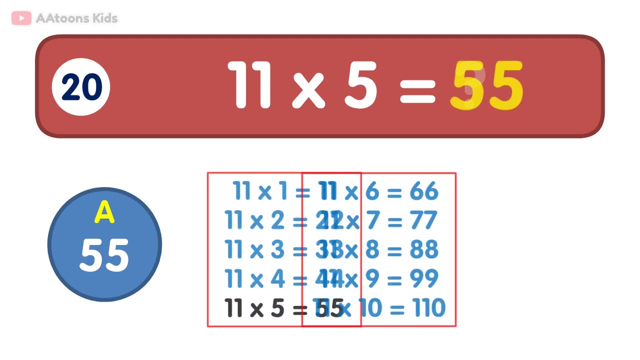 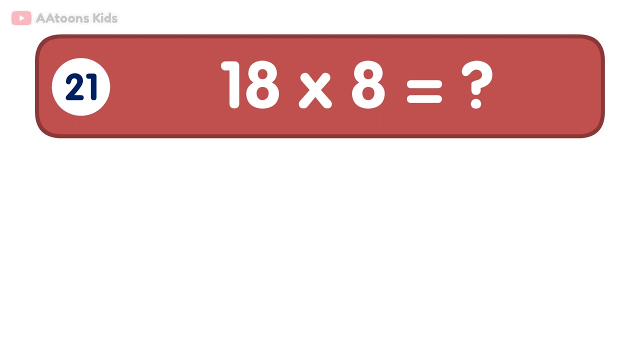 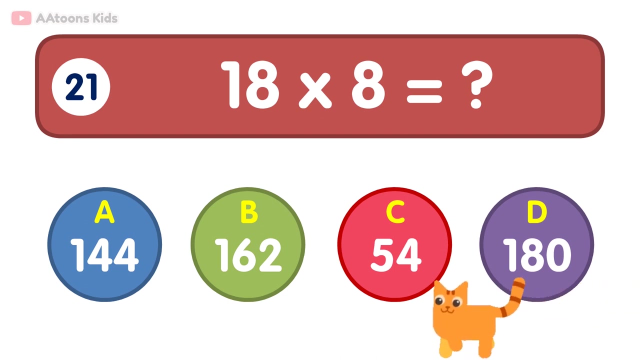 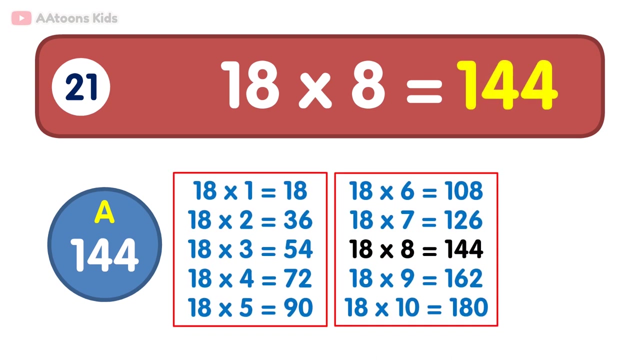 15 times 9 is equal to. 15 times 9 is equal to 55.. 11 times 5 is 55.. 18 times 8 is equal to 144.. 18 times 8 is 144.. 11 times 10 is equal to. 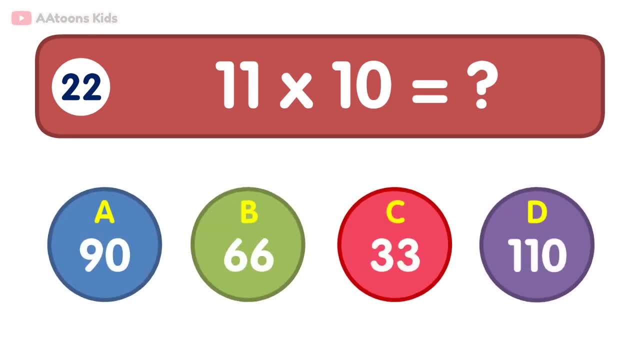 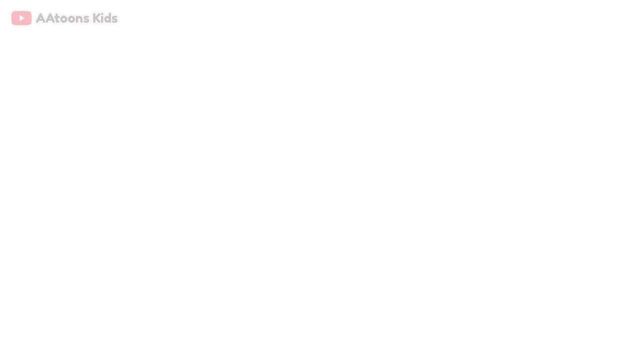 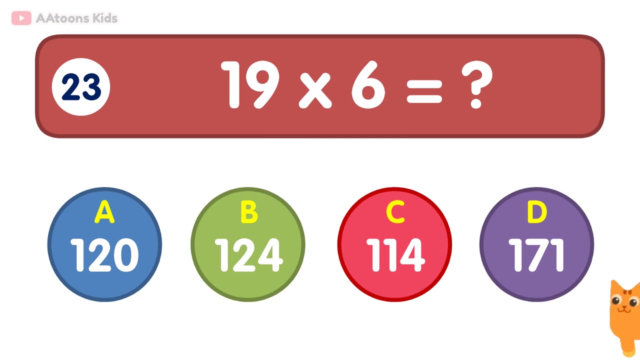 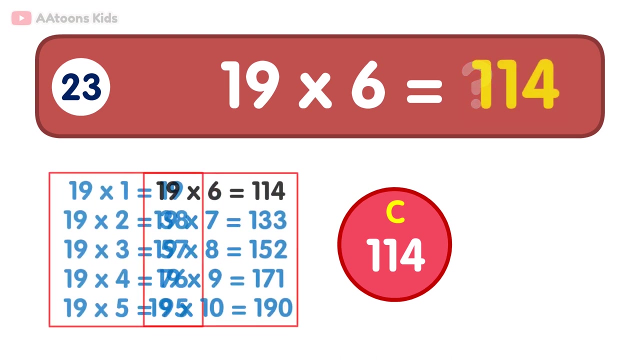 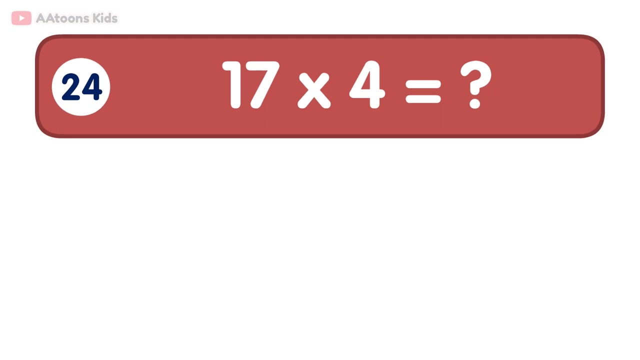 17.. 11 times 10 is equal to 18.. 17 times 8 is equal to 110.. 11 times 10 is 110.. 19 times 6 is equal to 11.. 114, 19 times 6 is 114. 17 times 4 is equal to. 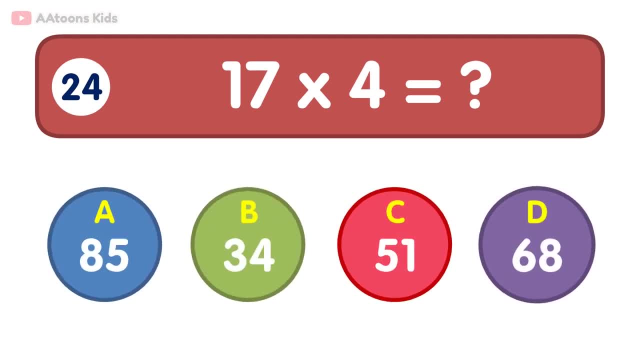 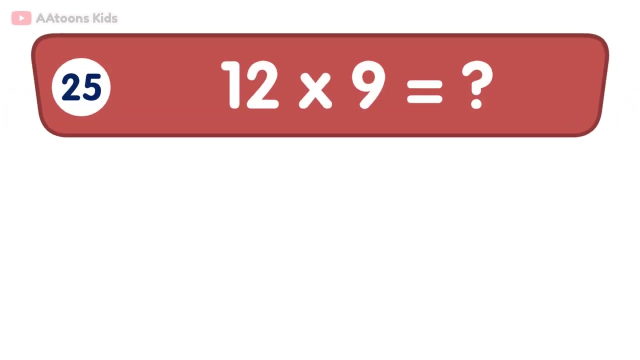 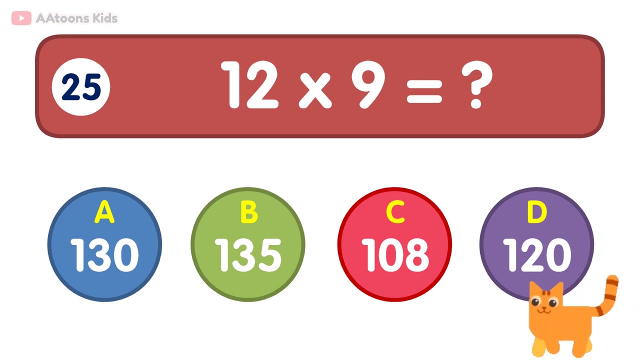 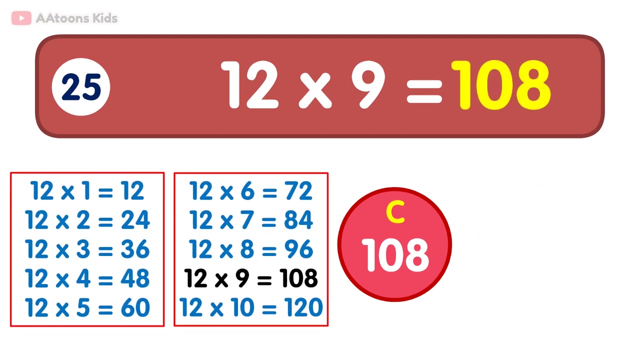 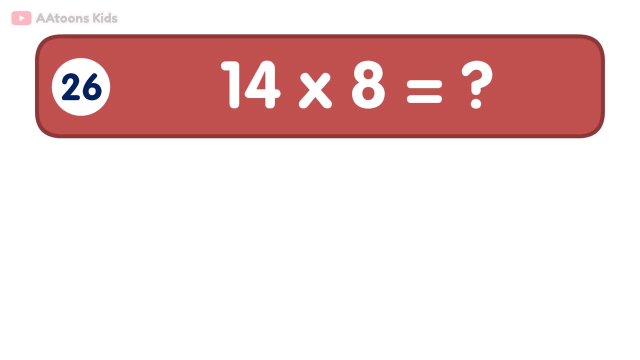 68, 17 times 4 is 68. 12 times 9 is equal to 68,. 17 times 4 is 68. 12 times 9 is equal to 108,. 12 times 9 is 108. 14 times 8 is equal to. 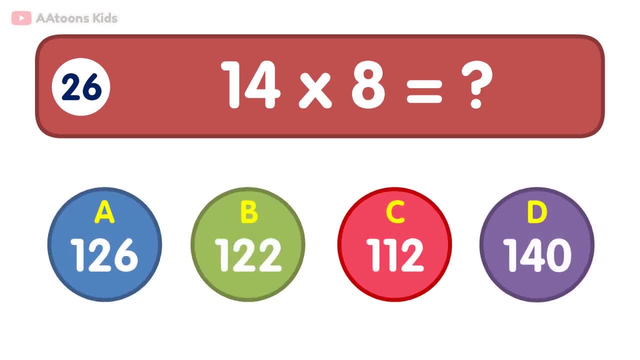 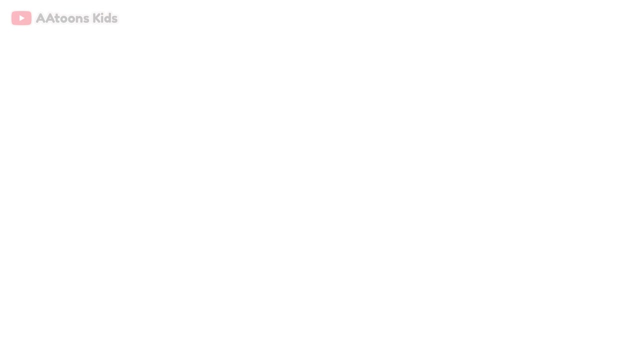 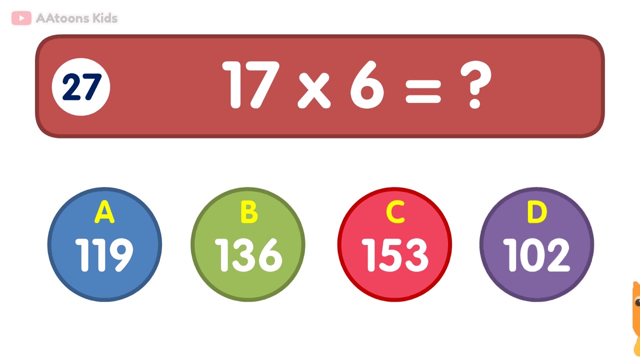 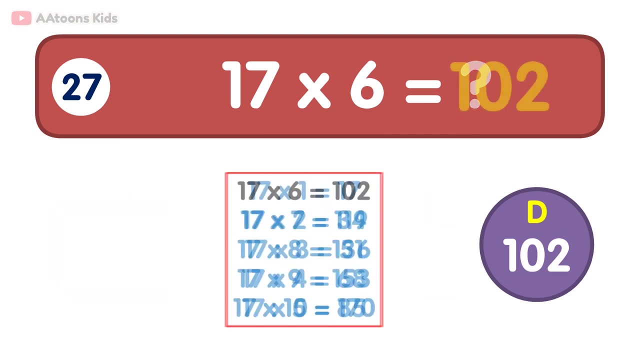 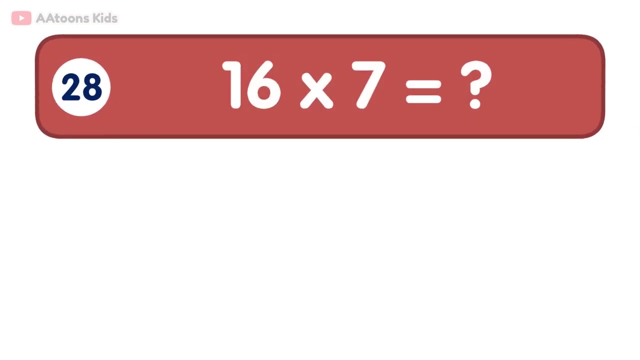 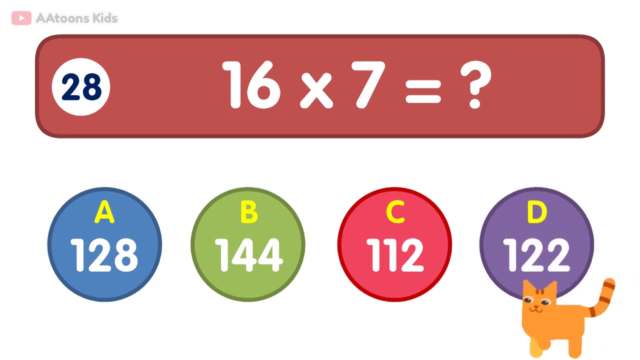 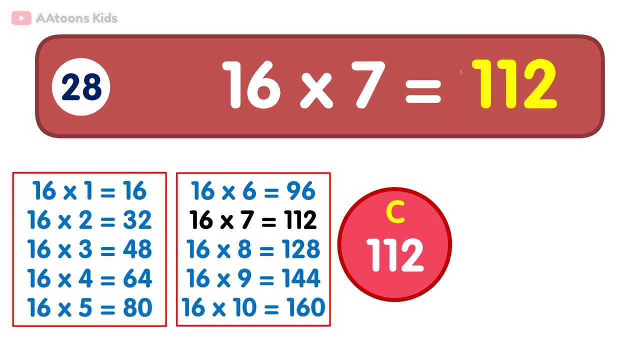 112, 14 times 8 is 112. 17 times 6 is equal to 12.. 14 times 8 is 112.. 102, 17 times 6 is 102. 16 times 7 is equal to 112. 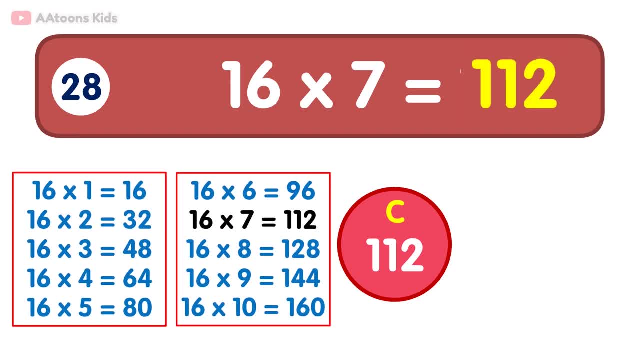 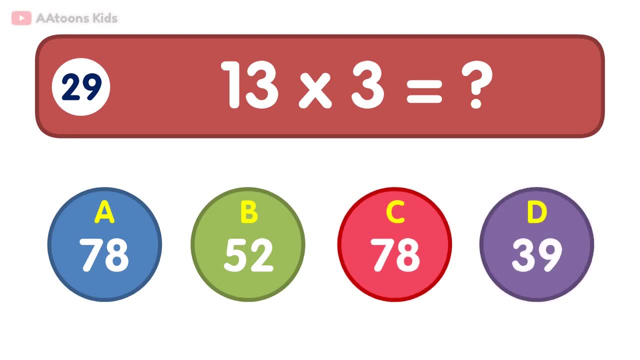 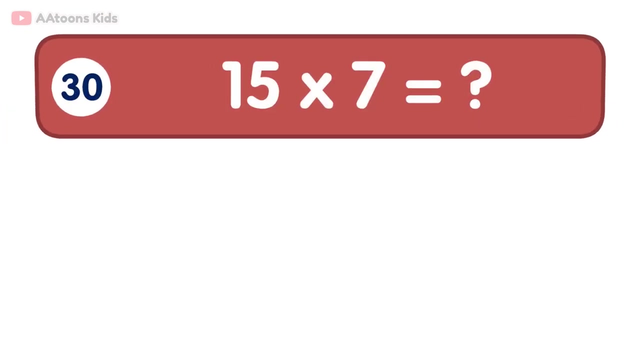 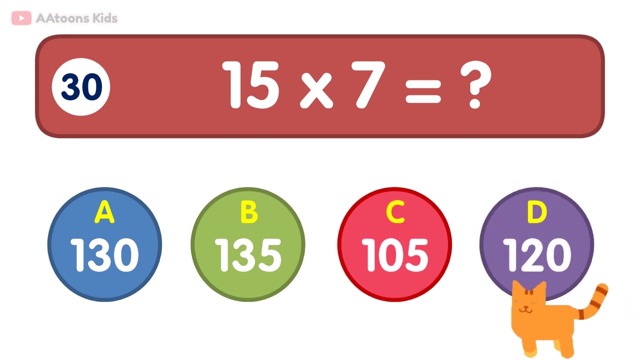 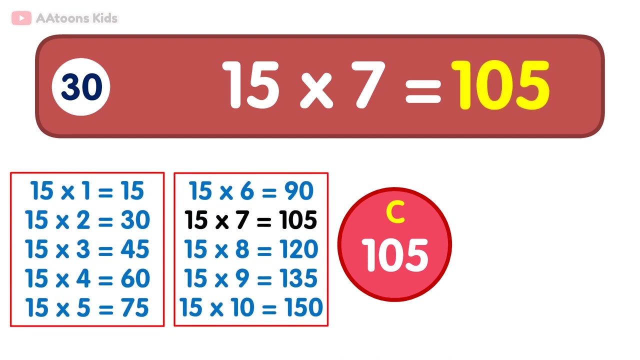 16 times 7 is 112. 13 times 3 is equal to 113. 39 13 times 3 is 39. 15 times 7 is equal to 16 times 7 is 105. 15 times 7 is 105. 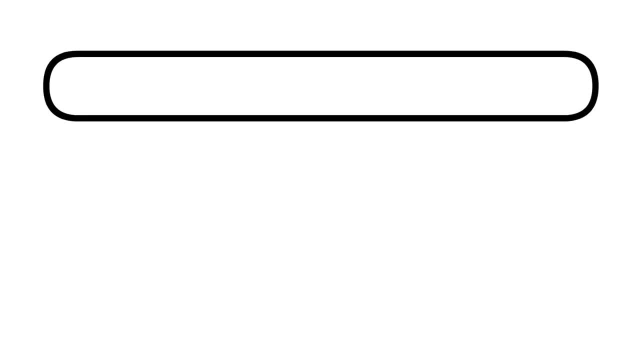 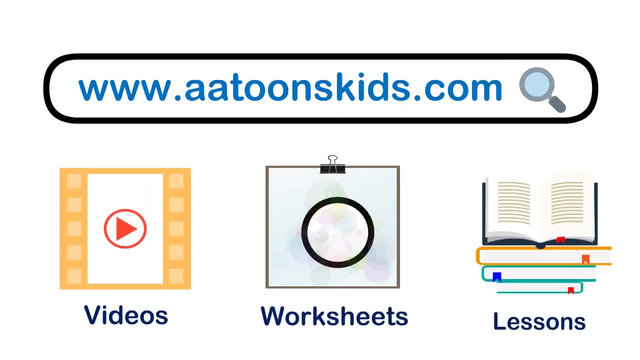